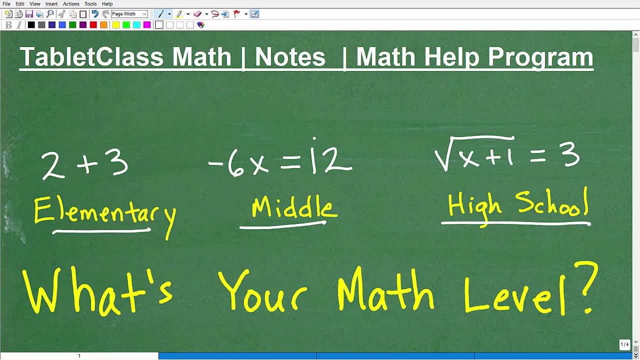 This is not absolutely precise, but I think it might give you a fair indication of what level you might currently be. Okay, that doesn't mean you have to remain at that level. You can always do things to learn and get to any level of math. 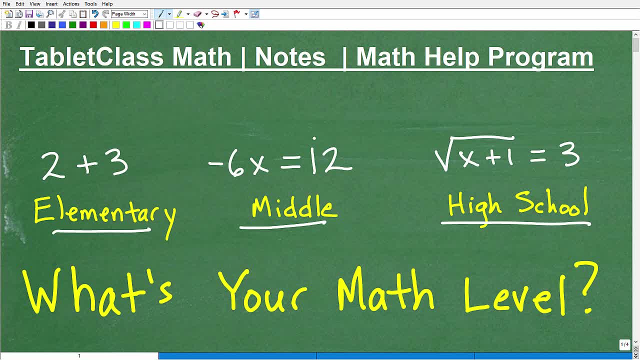 You want to. Okay, so we'll have fun with this in just one second. But first let me quickly introduce myself. My name is John. I'm the founder of Tablet Class Math. I'm also a middle and high school math teacher And over several years I've constructed what I like to believe is one of the 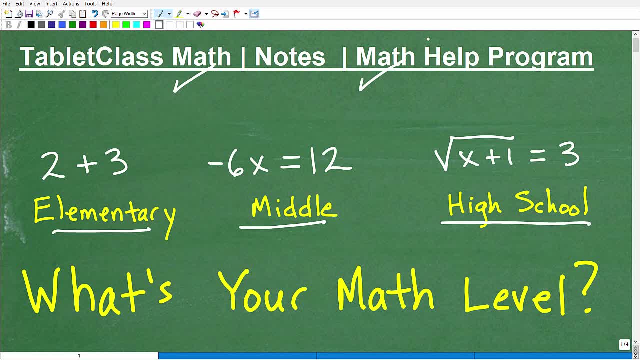 best online math help programs there is. So if you're interested, I'll let you be the judge that you can check out my math help program by following the link in the description of this video. But basically I have 100 plus different math courses ranging from pre algebra. 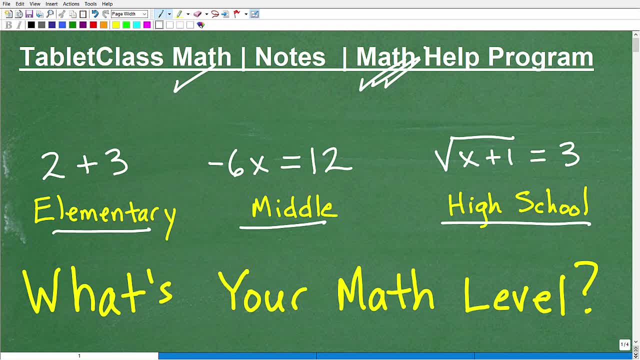 algebra one: geometry. algebra two: I'm going to be launching a pre calculus here, excuse me- in about a week. Very excited about that. I also do a lot in the area of test preparation. So if you're studying for the GED, SAT, ACT, GRE, GMAT, ASVAB, ACCUPLACER, ALEKS, maybe a teacher certification exam. 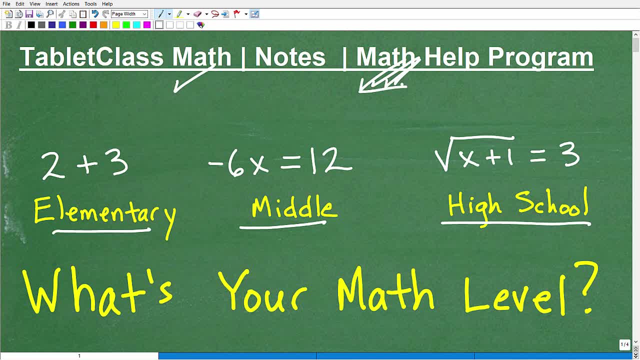 many other type of exams. I can help you out. Just go to my site, check out my full course catalog. If I don't, for some reason, have your exam that you're studying for, By the way, these exams, and a lot of exams, have math on them, Okay. and if you don't know, 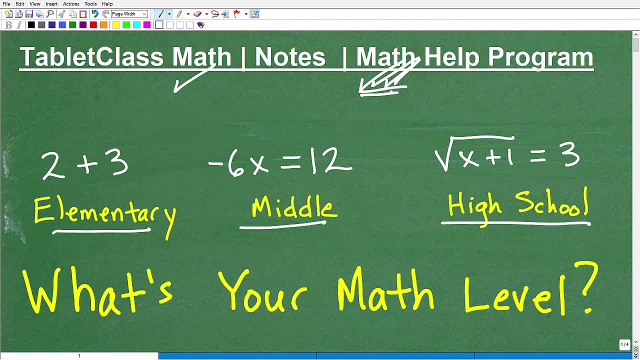 math. you're not going to do well in these exams, So I can really help you out with this. Again, if I don't have your exam, just drop me a line in my contact form And I will help you out. I also do a lot with homeschooling, So if you homeschool, I have a great homeschool. 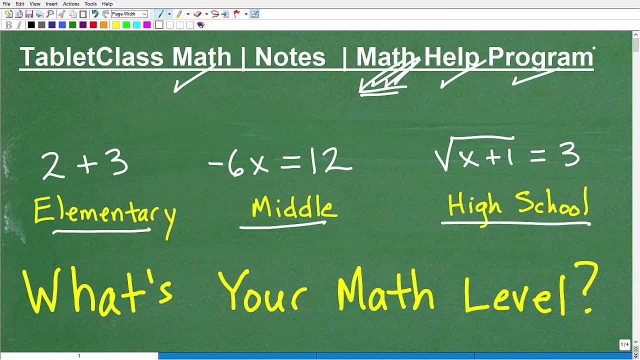 program And then obviously help those of you that are just having a tough time in your current math courses. Now, if you're truly serious about wanting to improve in mathematics, then you got to be serious about this. You got to take great math notes. There's just no way around it. So I've 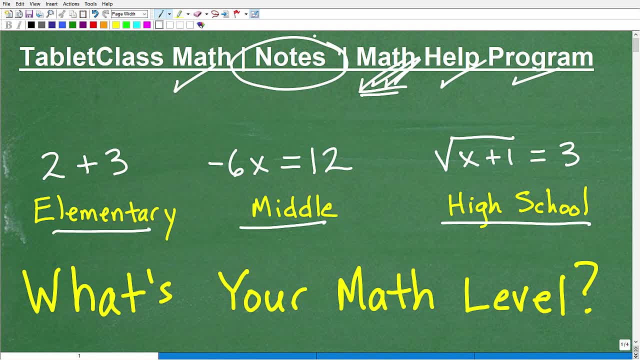 been teaching math for decades And this is the one thing that I can point to consistently: that when those students, when students take great math notes, they do very, very well. And the reverse is true, Those students who are like me, way back in good old 1986. 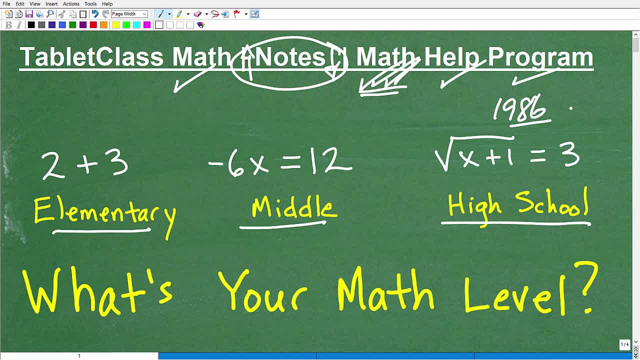 And what was I doing in 1986?? Well, I was in probably some algebra course taking notes, but they had nothing to do with math. I was like, hey, what are we doing this weekend? Well, guess what? you know, I didn't do too well in terms of my grades, And if I had a cell phone? 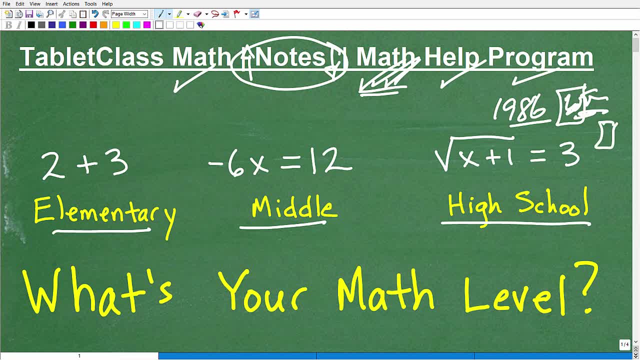 back in those days, I probably wouldn't even graduate. I wouldn't even graduate, I wouldn't graduate. So you're constantly distracted And I get that Okay. However, you're going to have to do whatever it takes to remain focused. Focus is the key to success, And that's a discipline. 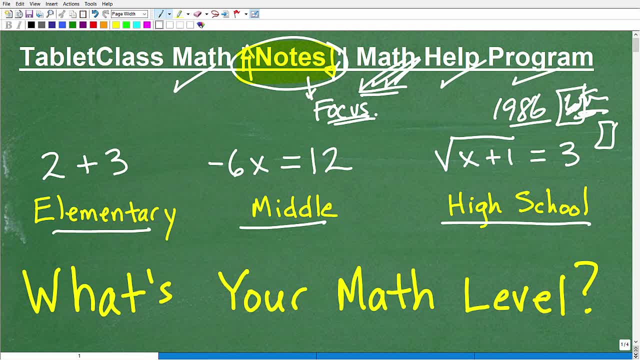 You're going to really have to work on that, But if you do that, everything else will become easy. Now, as you are improving in your note taking, you could use my notes to study. So those would include pre-algebra, algebra one, geometry, algebra two and trigonometry. You can find 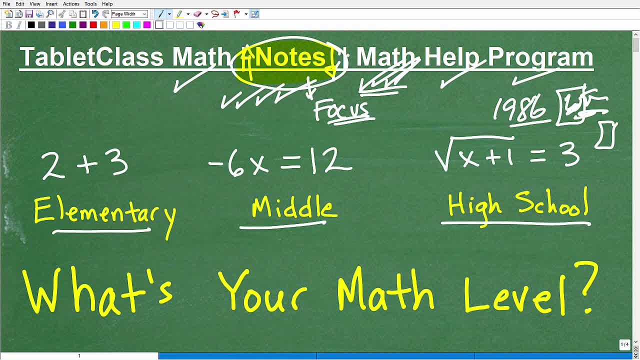 the links to those notes in the description of this video as well. Okay, So here we have three categories. These problems we're not going to do these particular ROMs, These are just kind of illustration of what would be at these various levels. So elementary math. 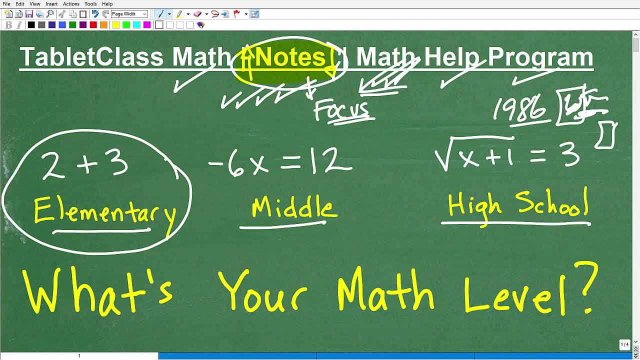 what do you learn? Well, you learn a lot of arithmetic. Okay, That's very, very important stuff. So, and there's quite a bit to learn. you know, in those, those developmental years, primary school, If you think about it, you're learning addition, division, subtraction. 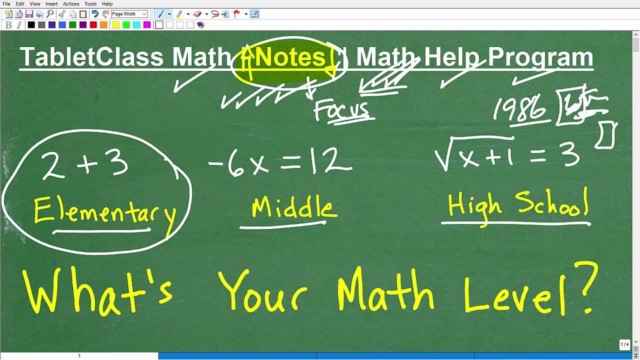 multiplication, your times tables, you know fractions, place values. There's a lot taught in here, So you don't want to just be like: Oh, you know, um, you know all, I, um you know. I'm just currently at the elementary school level, so I don't know much math. 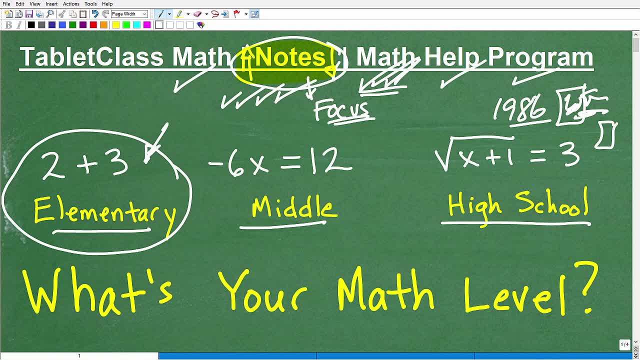 Actually, if you knew everything that was taught at the elementary school level, that's pretty good, Okay. So that's a good foundational start And certainly you need this to do well in middle school. Now, in middle school, you start learning um. you start learning about positive and negative numbers. 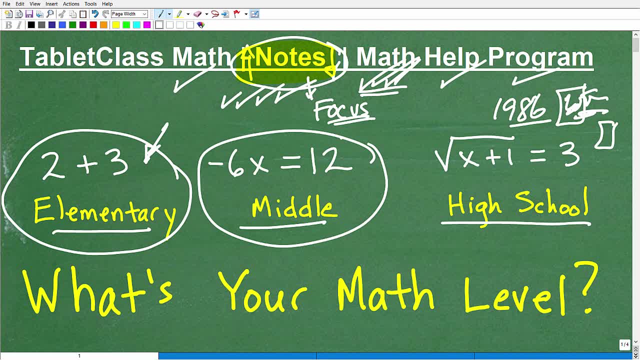 and you start mixing that in with positive and negative fractions and you get an introduction to algebra as well And you start doing more with geometry. Okay, So, uh, by the way, I've taught all these grades except for elementary school. I was not an elementary school teacher, but I've worked. 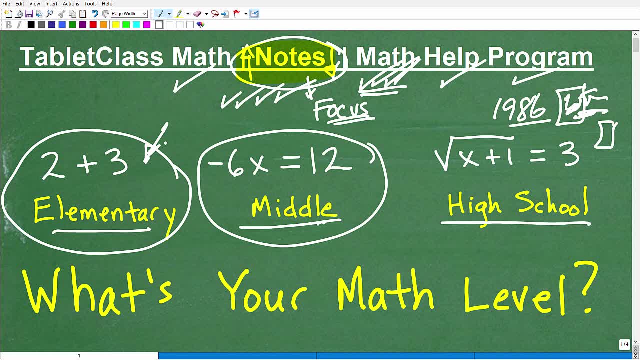 with a lot of elementary school teachers, because it's kind of like a- uh, a relay race. Okay, Students, when they graduate to elementary school, we pick them up in the middle school, Then we- uh, you know- graduate them on to high school. Now in high school, 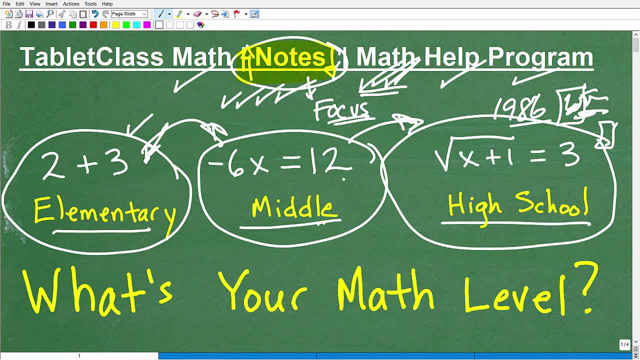 what are you doing in high school? Well, uh, if you get through middle school, this kind of leads- algebra- Okay, Basically, you should be doing a light version of algebra, but in high school, this is where things get really serious, So you're going to be doing algebra one. 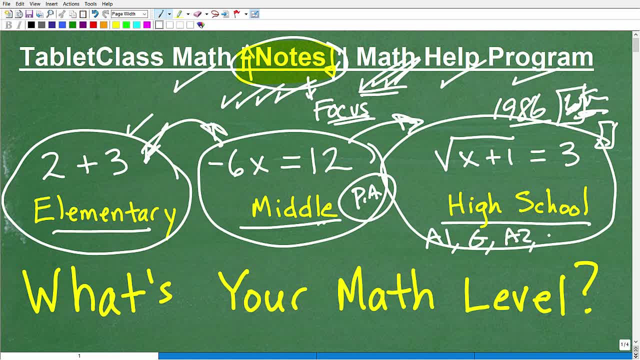 typically for most students, algebra one, geometry, algebra two, and then like pre-calculus or statistics. And if you were a superstar and started geometry in the ninth grade, you couldn't even be taking calculus um AP as a senior. So, uh, it all depends um. you know how you did in. 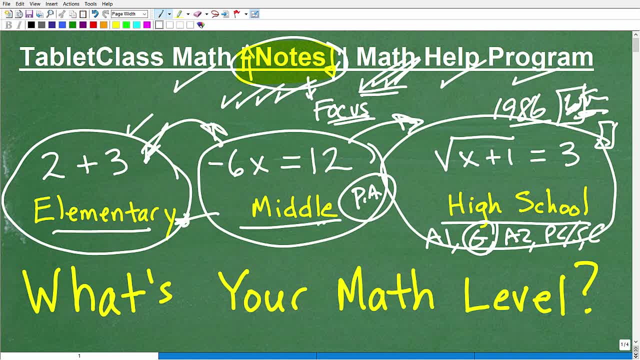 middle school, and how you did in middle school all depends on how you did in elementary school. It's all interconnected. But uh, anyways, let's have fun with this and let's see if we can get a basic idea of your current math level. Again, not your math potential, not what you can learn. 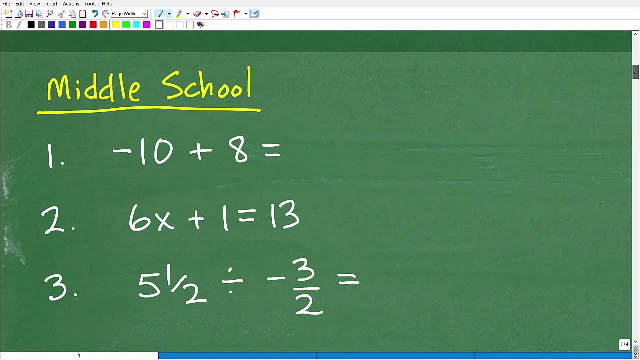 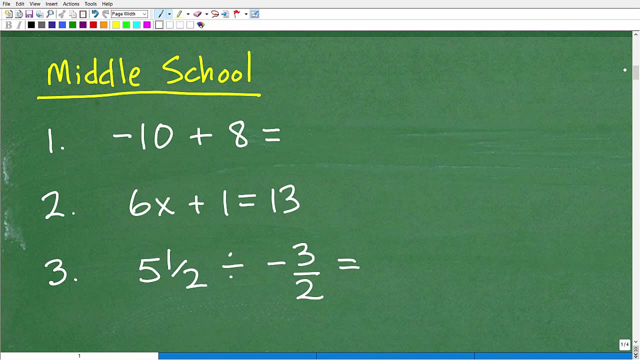 just kind of where you might be at All right, So I'm going to start off with middle school, because if you can't get these right, then let's just assume then you're at the elementary level. Okay, So that's the way I'm going to kind of do it. All right, So I've got three little 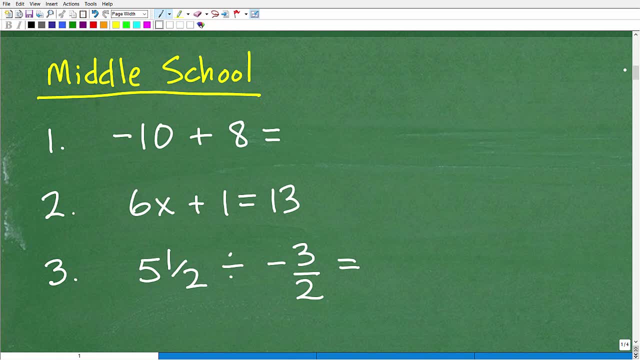 questions here. I'd give yourself about all of uh, geez, I don't know- 60 seconds, uh, one minute to go ahead and pause the video and see if you can answer these questions. Okay, If you get all these right, I would say you, you're okay. I mean, I would definitely put you in the 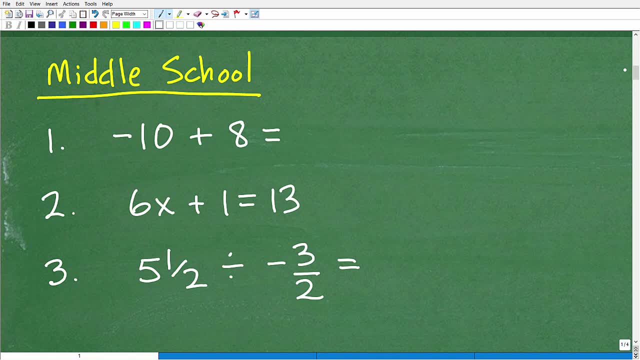 middle school range, And then I got some high school questions. but, uh, you know, if you can get these right, you're. you're beyond um, you're likely beyond elementary school, Okay. So if you want to hear the answers yet, pause the video. Okay, So number one now. by the way, um, here's. 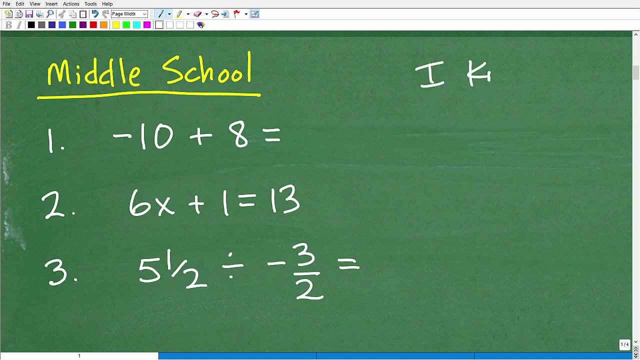 our answers. The one phrase that I, you know, will not accept- and you can just shut this video off right now and be like this guy's, giving me a ultimatums- is this one: Oh, I knew that, I knew. 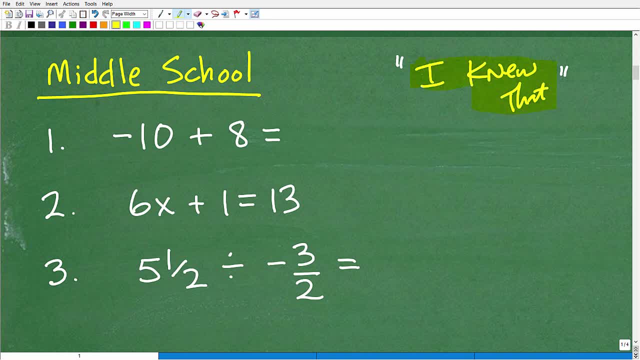 that, Okay, So you can't say that here, right? You can't say, oh, I knew that. So, in other words, if you get the wrong answer, but you, you knew what you're like, I see, you, see me do the right. 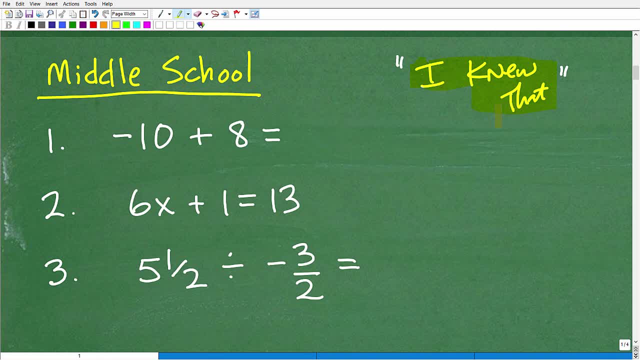 answer. but you did the wrong answer. but you say: I knew that that doesn't count, Okay, So this is. you got to know this stuff, but I do love that phase. I know that, I know that, I know that Well. 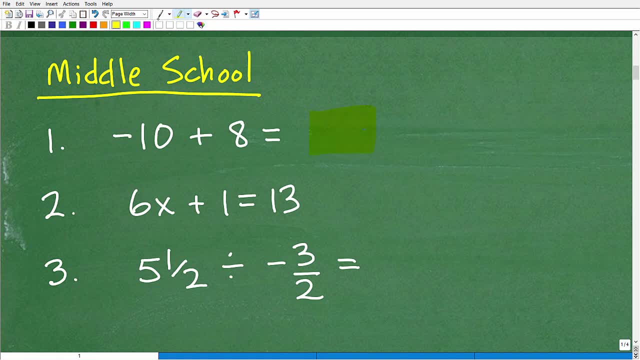 if you know that you got to do it. Okay, Let's get to number one. What is the answer? Drum roll, please. This is negative two. All right, So if you got that, that's excellent. Let me give you a. 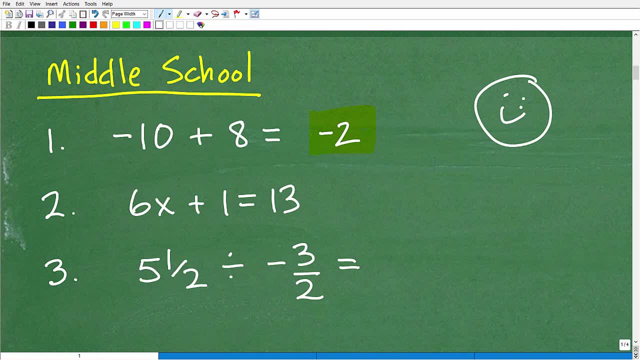 little smiley face. Um now, I know smiley faces aren't cool in middle school, but listen, I can give you one anyways. All right, Now I'm not going to explain to you about this, but I will make a comment. in middle school, You definitely need to know how to work with positive and negative. 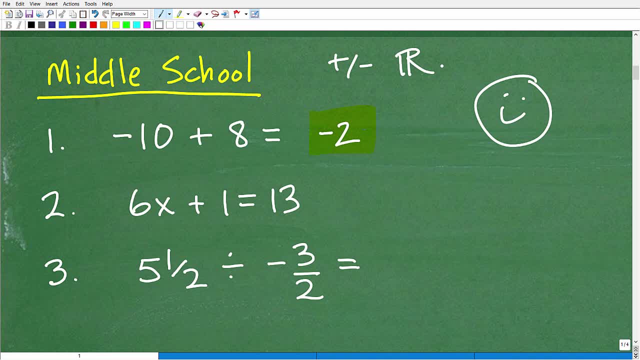 numbers. We call this the real number set. So we're talking about adding and subtracting, multiplying, dividing. It's not that difficult, By the way, in any of this stuff here. I have tons of videos on in my pre-algebra playlist. You can learn all this stuff All right. So this is not 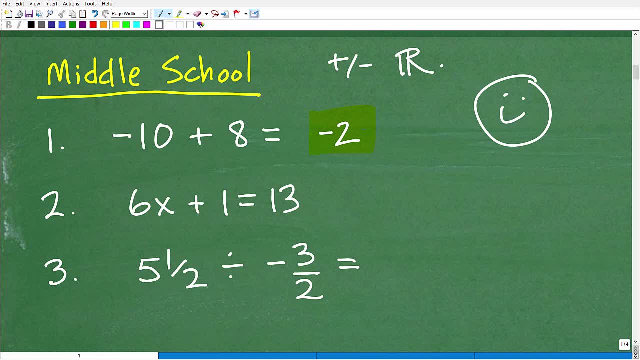 beyond you, but again, we just want to see what your current level might be. All right, Let's take a look at this uh equation. This is a basic algebra equation for number two. I'm going to solve it and you can kind of see if, in fact, you got the right answer. So what do we got? We got. 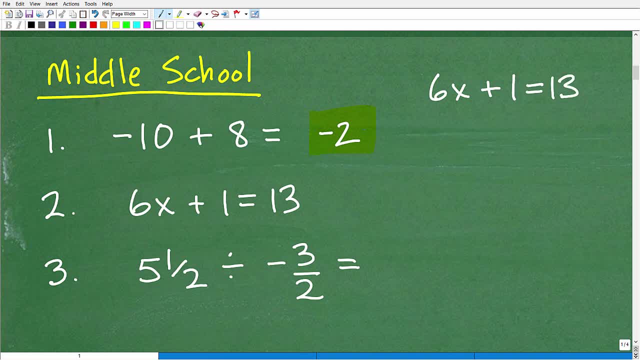 what we call a two-step equation, because it requires two steps to solve it. So we're going to solve All right. So what's the first thing I need to do? I need to subtract one from both sides of the equation. So it looks basically like this: I'm going to add down, I'm going to get six. X is 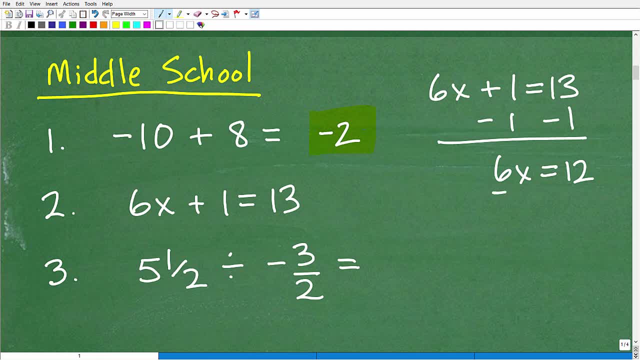 equal to 12.. Okay, And then I need to divide both sides of the equation by six and I get X is equal to two. So this is the answer here: X is equal to two. If you got that right, that's excellent. 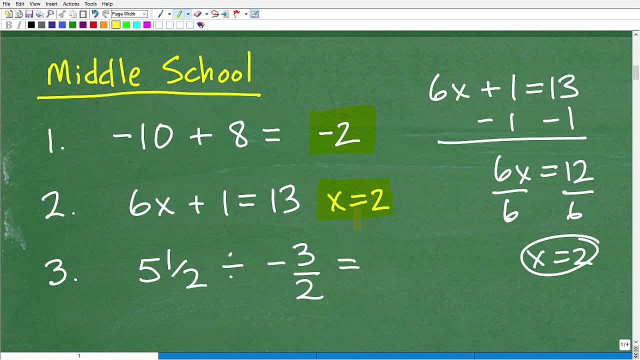 Okay, That shows me that you know how to solve basic linear equations up to two steps. And again you're kind of doing: you know pre-algebra, Then when you're in a real complete algebra, one course you do a multi-step equations right. All right, I would say, if you got these two. 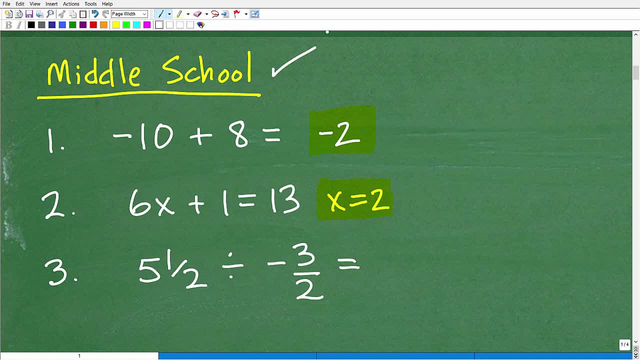 right, I would put you already in the middle school level. Okay, Now let's take a look at this. um, last problem. Now it's a fraction problem This have. we do have a negative fraction here, So that's why I kind of threw this in. So this might be, you know, um, if you don't get this. 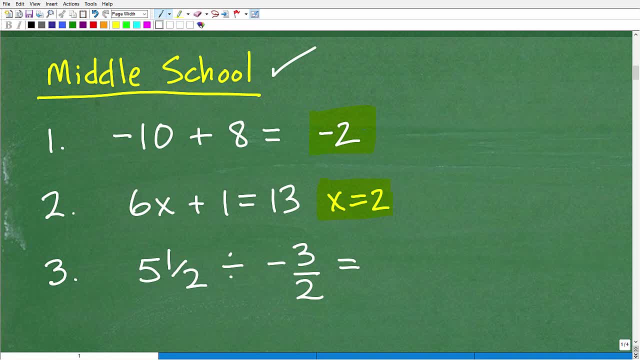 uh, think about, um, what you learned in elementary school, because we're learning a lot about fractions in elementary school, but here we have a division problem involving fractions. One of them is negative, This guy is positive. So what's a positive divided by a negative, right? 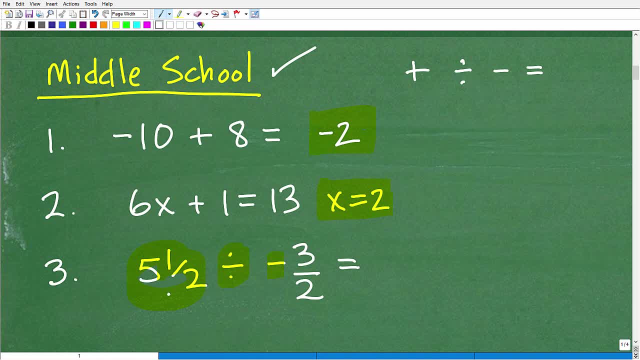 off the bat. Let's see if you can answer that question: What's a positive divided by a negative? Well, if you said negative, that's very good. Okay, So you're definitely at the middle school level. Now let's see if you can actually do the fraction problem. So 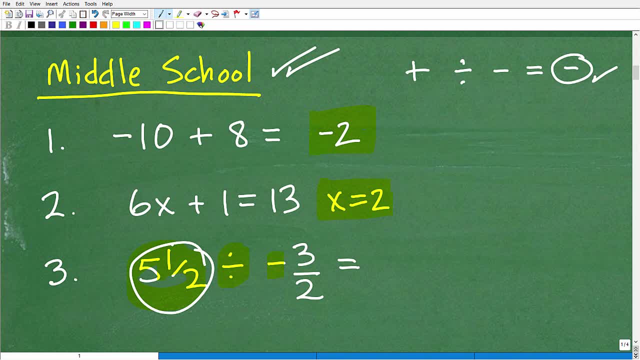 what you got to do here is you got to change this mixed number fraction into an improper fraction. So we go two times five, that's 10 plus one. So this is going to be 11 halves. Now this is division. We change that to multiplication and we flip this guy right And 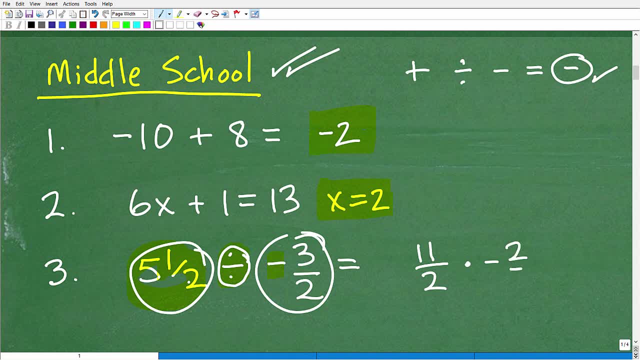 again. I'm not going to fully teach this. That's at the point of this little video. Okay, It's just a little quick diagnostics test. So it's here. So we got two times five, that's 10 plus one. 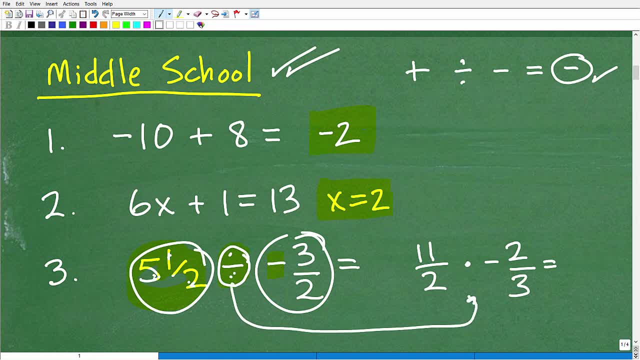 that's 11 halves. And then we're going to change the division, We're going to multiplication. That's how we divide fraction and fractions. And then we're going to flip this: This becomes two, this becomes three, And now we can go in and cross, cancel these. 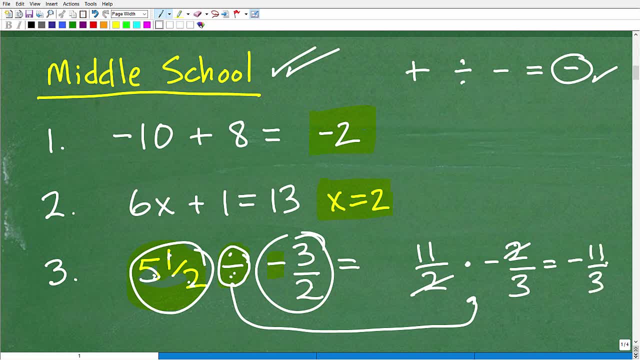 guys And this becomes a negative 11 thirds. Okay, All right. So if you got all three of these problems right, I would definitely put you firmly currently, right now, like between the sixth and eighth grade math level, which is very good, Okay. So obviously you got to know. 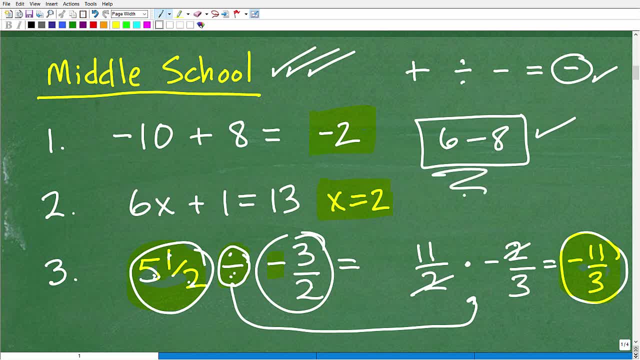 this stuff before you can really tackle high school level math right. But if you got these right outstanding Now, if you didn't, if you missed more than two, then you probably need to work on more. you know fundamental mathematics, taught in primary school, elementary school, but don't feel. 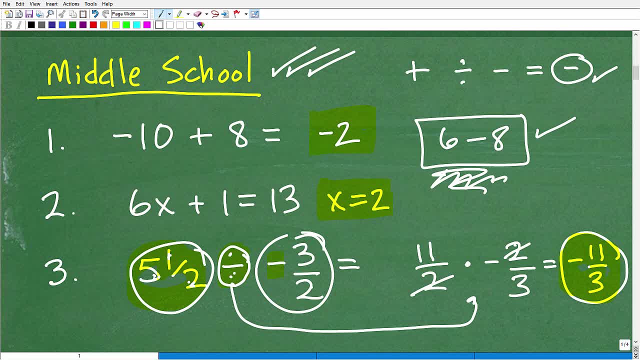 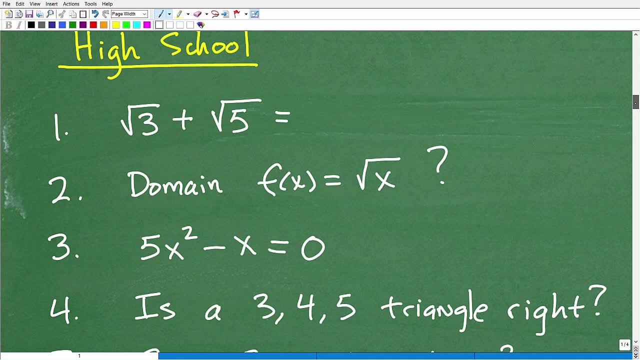 bad about that. You can just go back and review what you need to review, strengthen your foundation and then move forward. All right, Let's see if you are ready for high school math. So I've got some high school math questions here, and they're actually five questions. Let me show them to you. 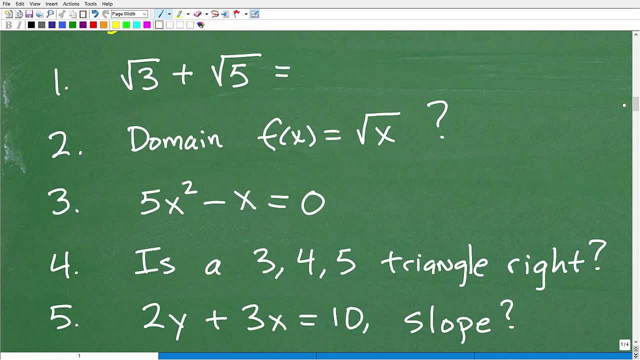 All right, So we've got number one. it's obviously. you know what this is. I'm asking you what the result is. This is number two. I want you to tell me the domain of this thing. Number three: I want you to solve this guy And number. 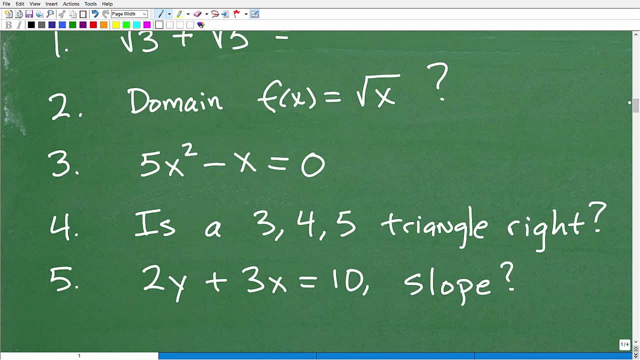 four. I want you to answer. the question is: three, four, five, Okay, These lengths of a particular triangle. Is this a right triangle? Okay, So justify your answer there. at number five, I have: two Y plus three. X is equal to 10.. This is a linear equation. I'd like you to tell me the slope of this. 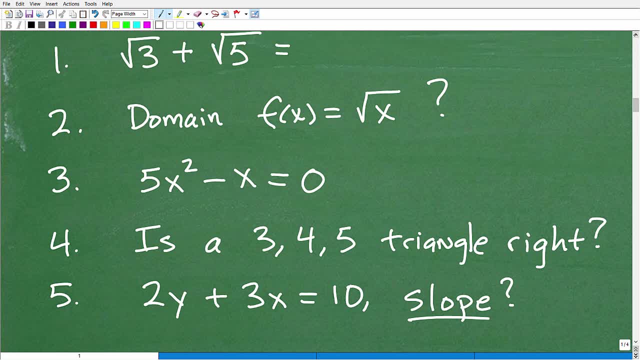 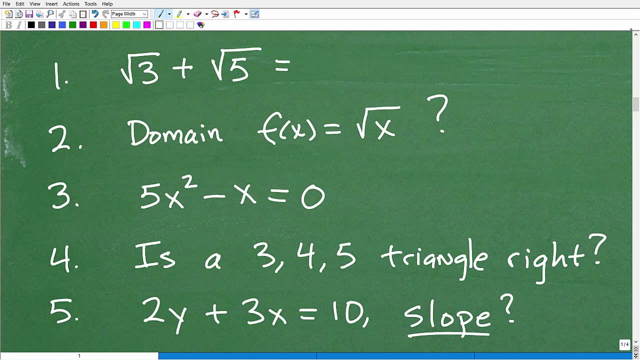 thing. Okay, All right, So these are the questions, And I would give you, give you, a good solid five minutes to answer these. No more than five minutes should be sufficient. Now I'm going to go through these things pretty quickly because I don't want to make this video too long. So, again, I'm not trying to. 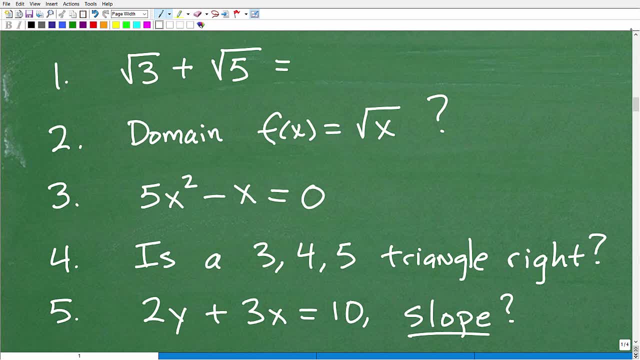 teach all these various topics and what you basically, you either know this stuff or you don't, Okay, But if you can get through all these and you definitely have a fairly decent you know you got your bearings with some high school Math. Okay, Now this is all inclusive. Well, this is kind of like at the algebra, one level, maybe a little bit of. 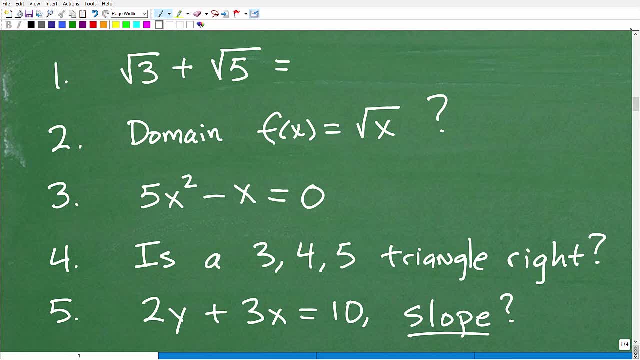 geometry, but you know, we're just having fun here. Okay, Where you certainly put- let me just say this much: If you can get these answers right, Or the majority is right- You're beyond middle school. You're definitely in the high school range. Okay, All right, I'm going to start answering these questions right now. 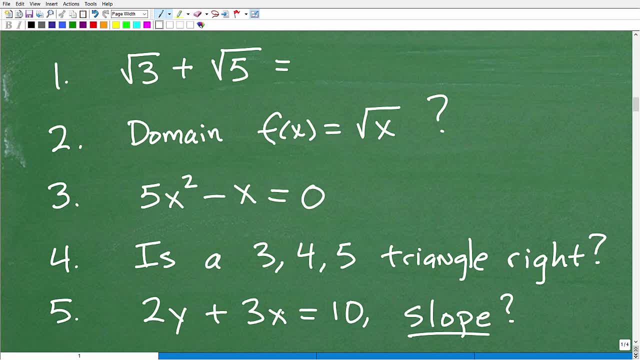 And so if you don't want to see the answers, if you're not ready for that, pause video and let's get going. Okay, Then remember the phrase. I knew that. I knew that That doesn't count. All right. So number one, square root of three plus square root of five, what is the answer? 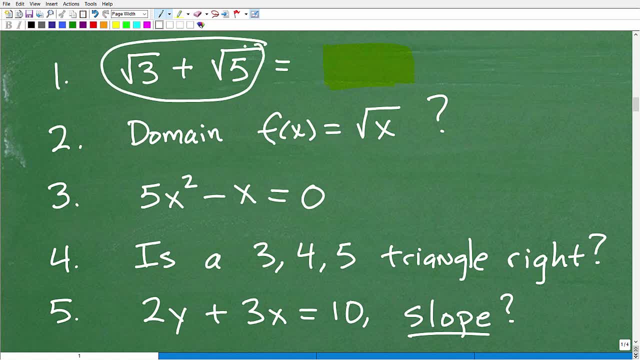 Well, this is the answer. Okay, We cannot simplify that anymore. So if you did square root of 15, I'm sorry to inform you- you get a sad face. All right, That's the one you're when you're multiplying, Okay. 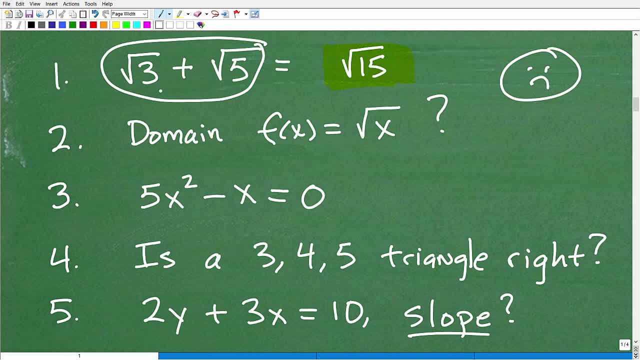 When you're multiplying radicals or square roots, then you can multiply, But when you're adding these things are like like terms. So this is not the answer. This is the answer. This cannot be. Uh, this is simplified and you might be saying: man, that's a trick question. 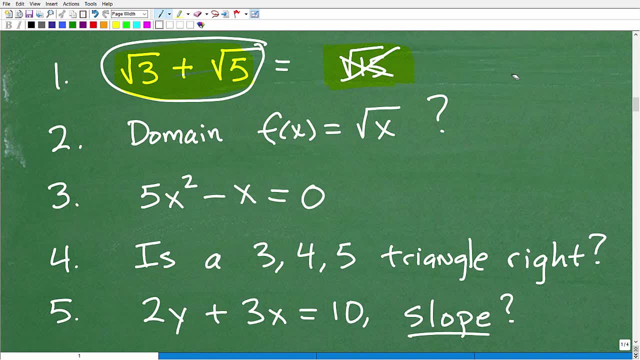 That's not fair. Well, listen, this is the way it goes. Okay, Let's talk about number two. We have a function again. Uh, we need to know what this word domain, uh, stands for or what it is. 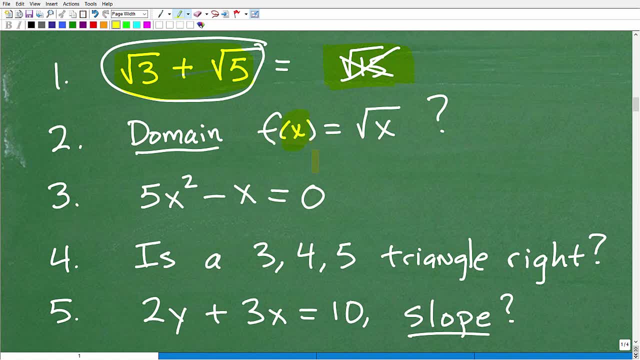 And basically that's the allowable input values into a function. Um, now here again. if you don't even know what I'm talking about, then don't don't panic. Just means that you need to. you know work on this topic, but functions are hugely important. 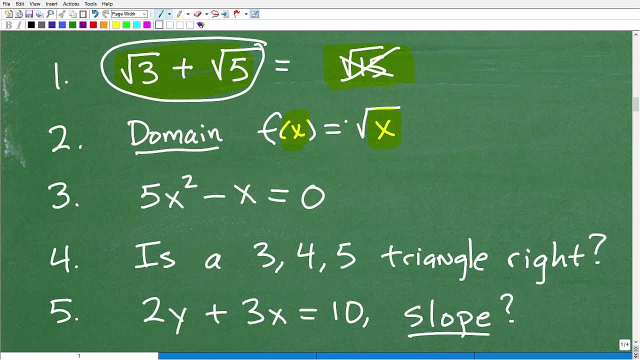 In algebra, which is, of course, you know, a huge part of high school mathematics. So the domain, okay, What I can plug into this function is: there's a number of different ways You can say this: all X is greater than or equal to zero. 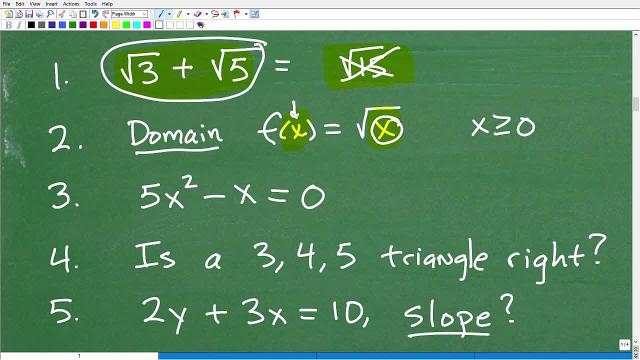 Basically I cannot put a negative number in uh to this function. So the domain. you could express it something like this: uh set of all real numbers, such that all X's are greater than equal to zero And X is a member element of the real number. 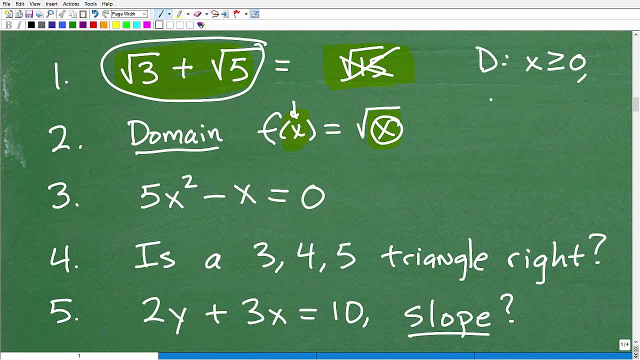 System is a bunch of different ways You can. you can do this. You could even do this: uh, zero to positive infinity. I don't really care, as long as you're saying you can't put negative numbers into this. That's what makes a difference. 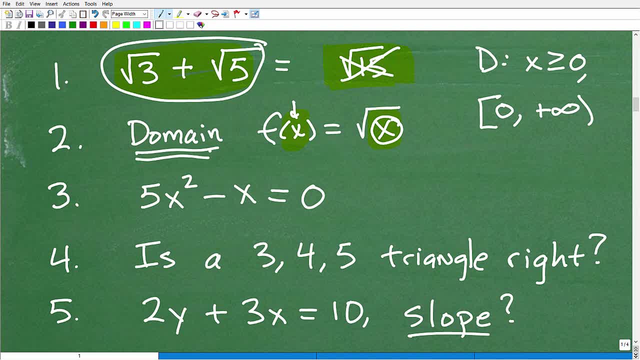 Okay, And if you understood the concept of domain, then you're good to go, All right. So if you got these two, uh right so far, and then that's that's pretty good, All right, let's take a look at number three. 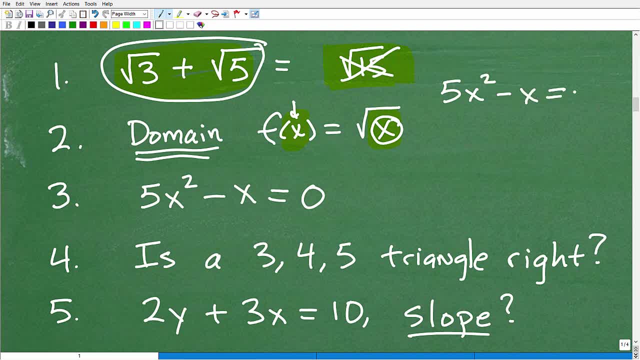 We got five X squared Minus X is equal to zero And, by the way, two. let me just mention. I have tons of videos on all these various topics, uh, uh, in my YouTube channel. Again, if you really, really want to learn this stuff, you might want to consider um taking one of my courses. my most basic course, uh, most basic course right now currently is pre-algebra. 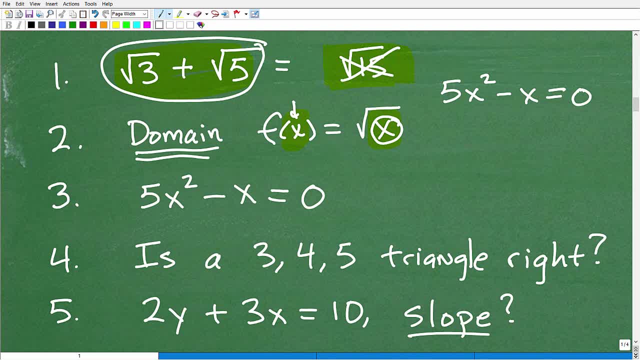 Okay, But uh, all this stuff would be within algebra and beyond. All right, So what do we got here? Well, this is a quadratic equation. There are two solutions. How can I solve this easy, I could just factor out at X. 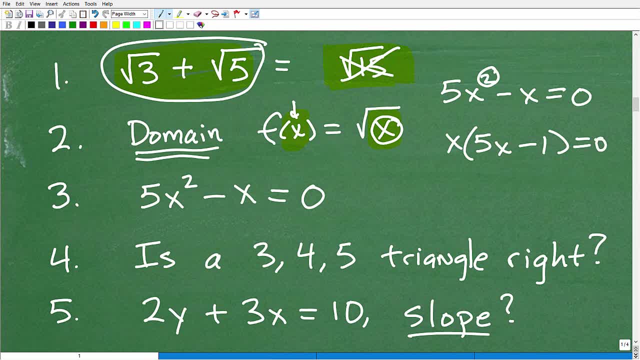 That's going to be Five X minus one. that's equal to zero. Okay, So if I distribute the X back in, I get five X squared minus X. here I have the factors, and this times this is equal to zero. 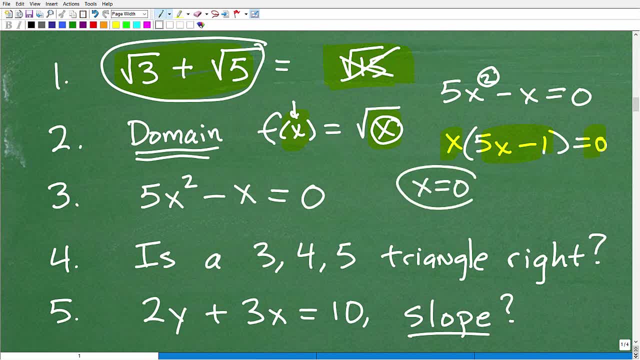 So I can set each factor equal to zero. So X is equal to zero, That's one solution. And five X minus one is equal to zero. That's going to be another solution. So I need to solve for X here. So I get five: X is equal to one or X is equal to one. 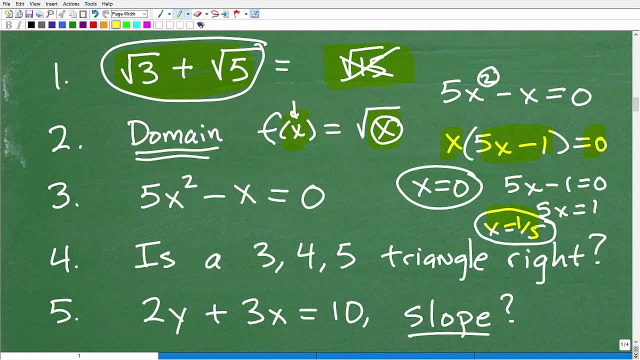 And that's one And one fifth, And I'm kind of run out of room, but that's basically it. So those are the answers. They're zero and one fifth. Okay, If you just only gave me one answer, that's not sufficient, because you need to know that there are two answers here. 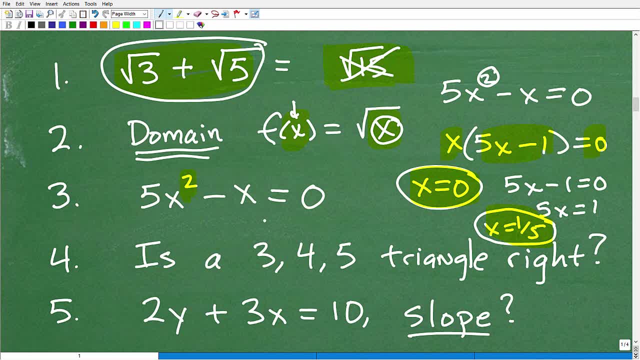 Okay. So if you got that one, that's pretty good, because this is a quadratic equation that shows me you know how to factor, You understand the zero product properties. This is, this is good Okay. So if you're up to these three guys, pretty good. 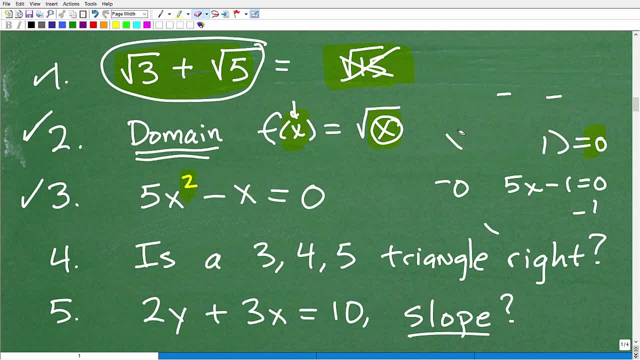 All right, Now let's erase all of this And answer the next question. All right, so is 3,, 4, 5 a right triangle? The answer is, in fact, yes, it is Okay. so how can I prove that? Well, if it's a right triangle, the longest side of a triangle. 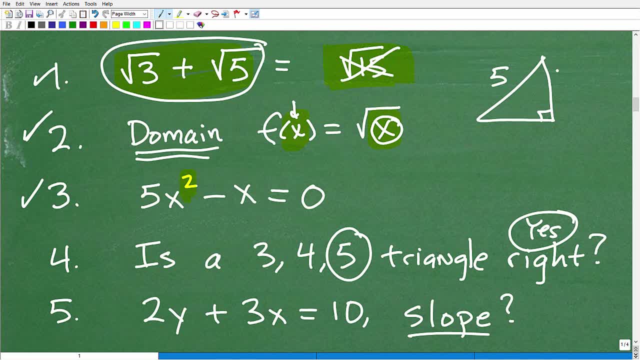 is going to be the hypotenuse, So this would be 5, and then 3 and 4 would be these legs. So maybe it's 3 and 4, and we can justify our answer, yes, by the Pythagorean theorem: a squared plus b. 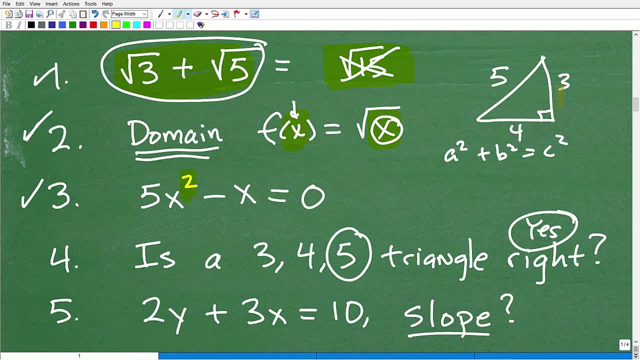 squared is equal to c squared, So a and b would be these sides. C is always the hypotenuse, So let's plug these in. So we have 3 squared plus 4 squared. Is that, in fact, equal to 5 squared? 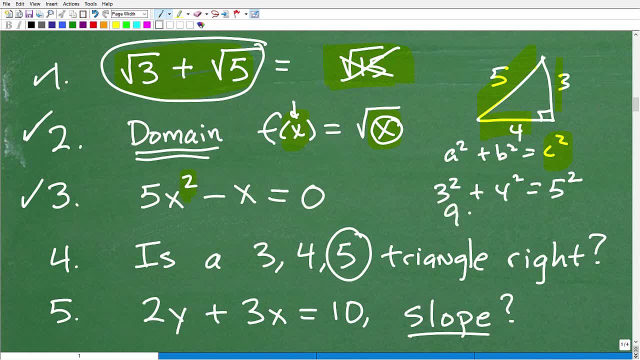 It is right. So 3 squared is 9 plus 4 squared, That's 16.. And 5 squared is 25.. Is 9 plus 16 25?? It is 25 is equal to 25.. So 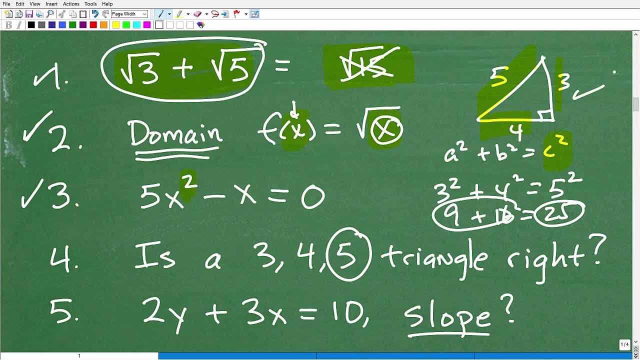 I don't know. That is in fact a right triangle. All right, so we got that right. That's very, very good. And let's finish up with this last question. Again, I'm just flying through these. These are some random questions. I could have put other ones, but if you're getting these, 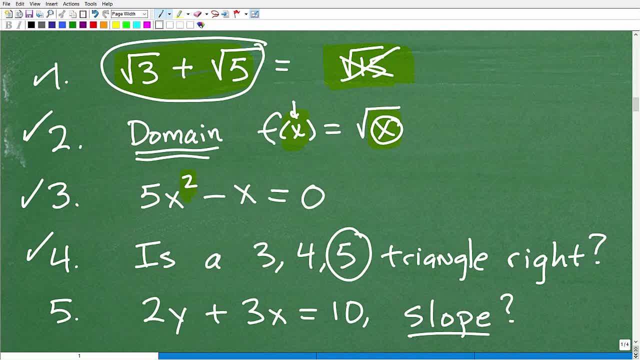 right, you're definitely in the high school level, okay, All right, let's go ahead and find the slope of this guy right here We have: 2y plus 3x is equal to 10.. The easiest way to determine the slope of this linear equation is to solve for y. So I'm going to do that now. I'm going to. 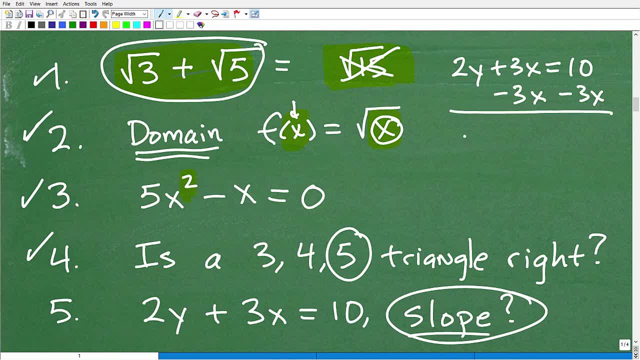 subtract this 3x from both sides If you don't know what I'm doing. again, that's not the point of this video. I have tons of stuff on this in my channel in my courses, But we need to solve for. 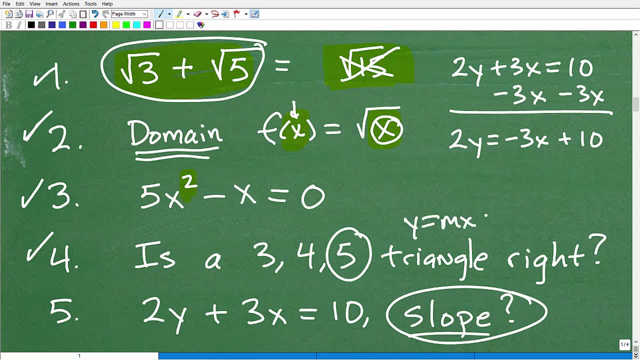 y, because I want to get this into. y equals mx plus b form, okay, And once I do that, I could look at the m and that'll be my slope. all right, So that's why I'm doing this And I'm almost there. 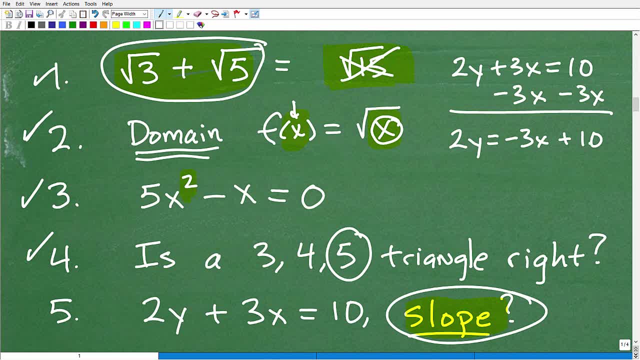 I have 2y equal to negative 3x plus 10.. Let's divide everything by 2 now And I end up with: y is equal to negative 3 halves x plus 5.. There's my linear equation in: y equals mx plus b form or slope intercept form, And this is my slope negative 3 halves. So if 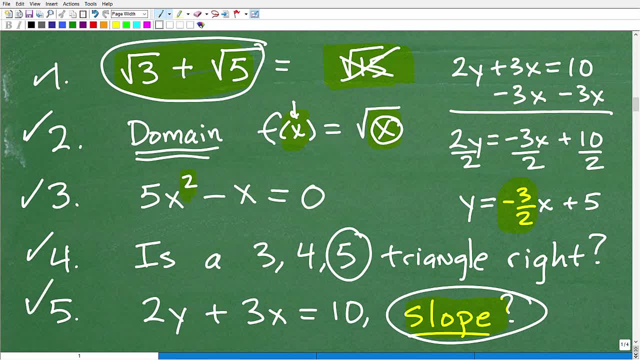 you got all of these right. I would say, if you got at least three of these right, if you got two, then I would, you know, think that, yeah, you're kind of like them would be in between middle and high school. In other words, if you got this right but you forgot this other stuff. 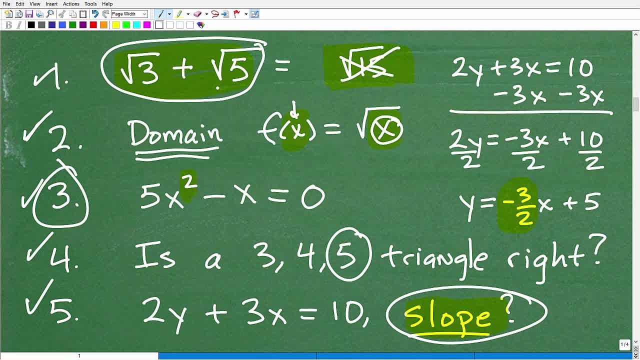 well, you kind of know, right, You'll. you know, I'm like I don't have to tell you, right, If you're like, no, I kind of knew this. I just need a quick review. You, very well, are probably beyond middle. 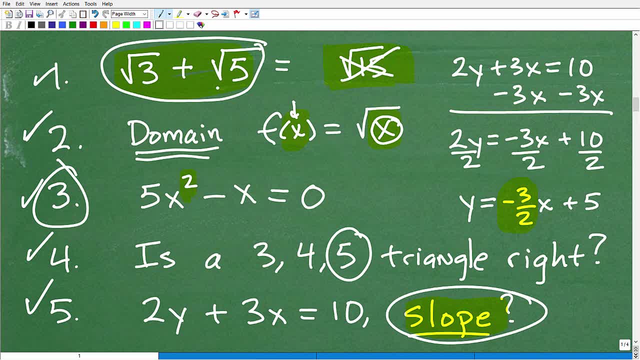 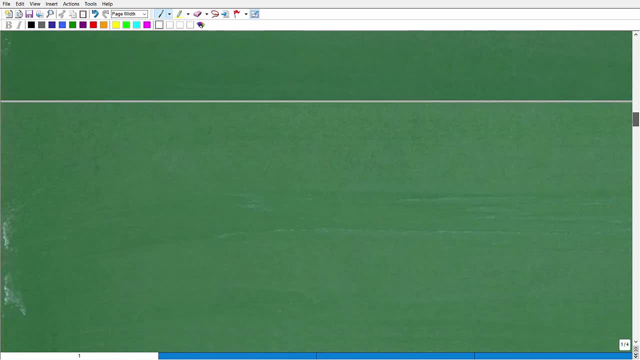 school. But if you got like three of these, three or four of these wrong, then you probably need to go back and brush up on your middle school math and start taking algebra. But if you got all these right, man, that's pretty awesome stuff right? So in let me go ahead and give you a happy face. 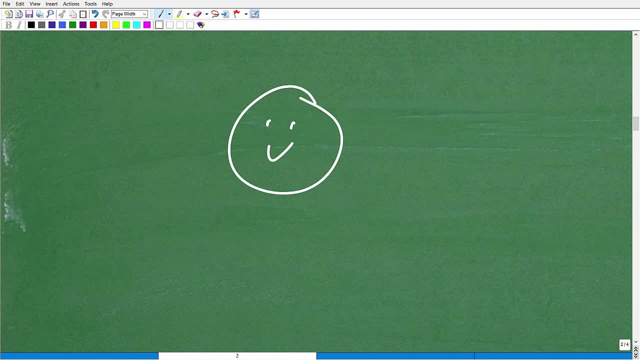 for no matter what level you're currently at, right. If you're at the elementary level- listen, don't panic. All right, that's, that's pretty good, Right? If you're at the middle school level or at the high? 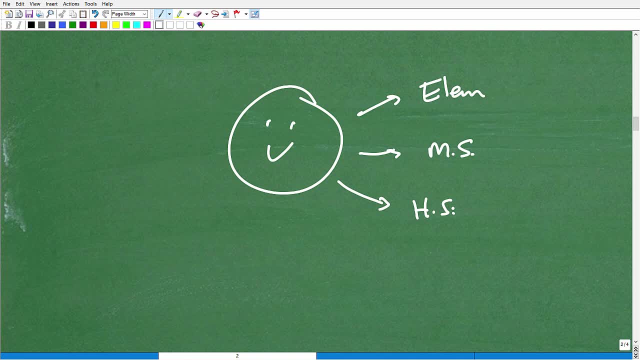 school level, it doesn't make a difference, Because learning math is about finding your starting point. All right, So here, this is the way I look at mathematics. Where do you want to go? What is your goal? Okay, Do you want to take calculus? Do you want to? you know, get a great. 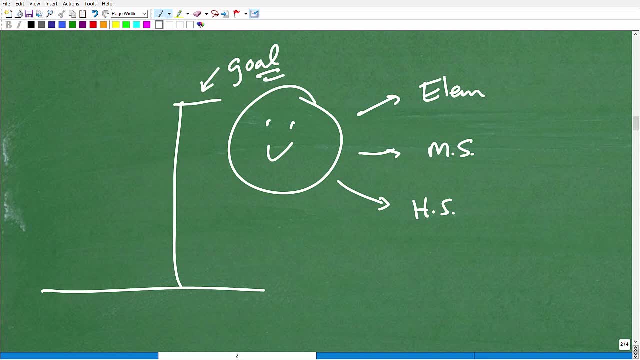 SAT score. I don't really care what your goal is, You know. you got to define where your goal is at And then you got to start basically taking some steps to get to your goal. Okay Now, if you're at the elementary level, all right, so what? Maybe you're starting at this level, but you're just going to be taking these steps anyways. If you're at the middle school level, okay, well, you're just starting at this point. you're still got to go up this level. And if you're at the high school level, maybe you're right here, but you're still going up. Okay, The bottom line is: you can't let you know your 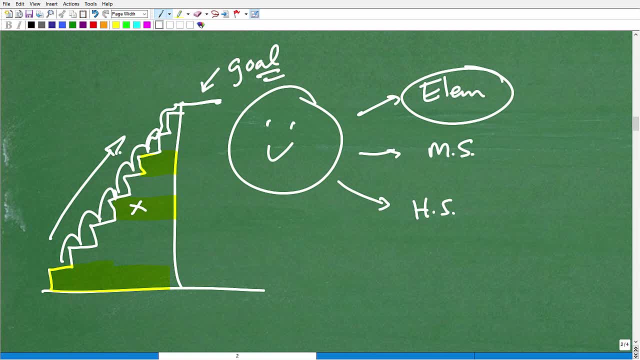 current math level, define your potential or you know what you're trying to accomplish. Okay, And, by the way, too oftentimes a lot of the students, especially like at the middle school or the high school level, think they've mastered the previous level And in fact they're kind of shaky at these things and they don't have a strong foundation. So as they get up here in more advanced mathematics they kind of like peter out And you know they find it very, very difficult because they don't have those strong foundations. So really build. 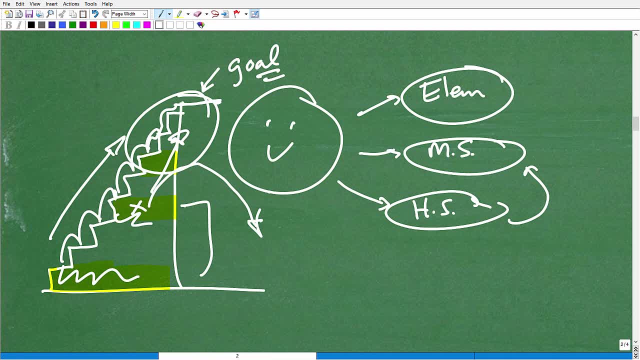 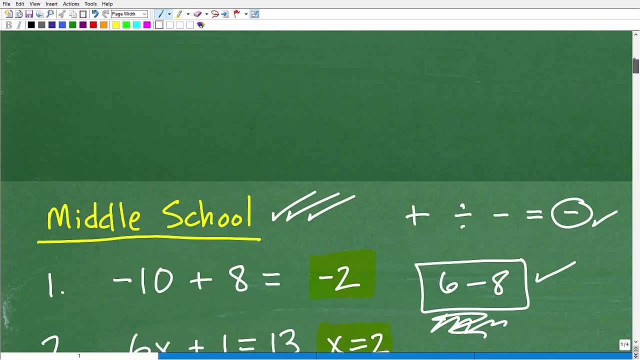 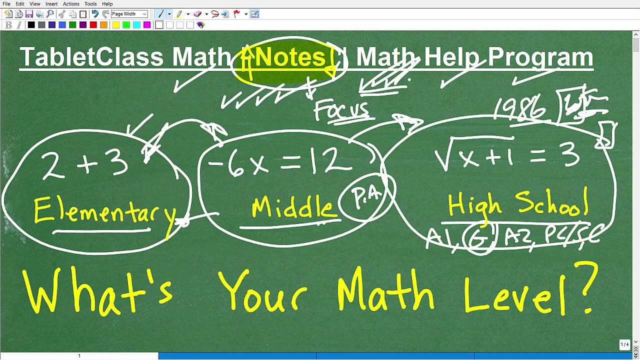 you know, up your math skills like one solid brick at a time. Okay, and you do that, you'll build yourself a nice fortress And I'd like to help you along with that little you know goal right, I mean, math is everywhere. right, Let's talk about all the tests that you have to take. These tests are a college placement test, vocational school, military. you know, you just can't escape math. Okay, It's everywhere. So, anyways, 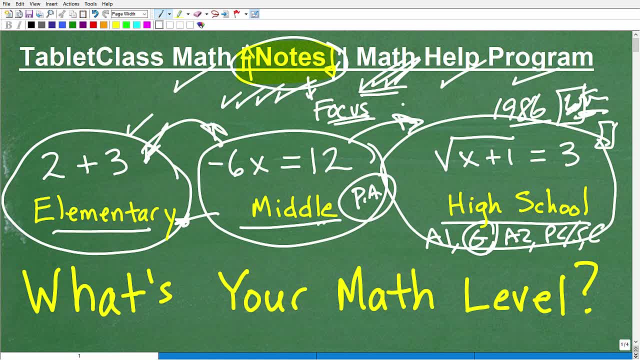 if this video was helpful in some way. if you're like: okay, well, at least I got some better sense of where I might stand, Well then please consider smashing that like button. That helps me out. And if you're new to my YouTube channel, please consider subscribing. I've been on YouTube for 10 plus years. I have over 1000 math videos, basic to advanced math. So if you like my teaching style, well, you can learn from me and I'll post new content all the time. But my best math help- if you really really want to, you know, increase your math skills and you might want to consider my math help program because that's my best stuff there.